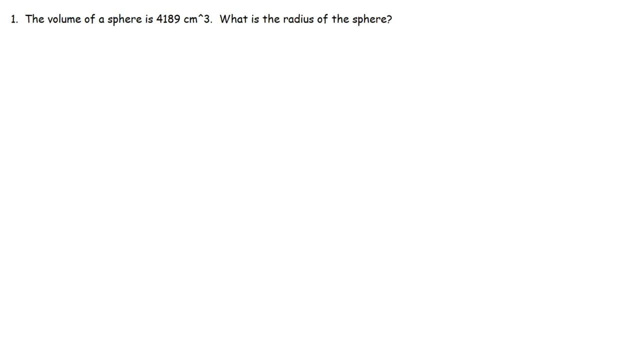 In this video we're going to talk about how to calculate the radius of a sphere, given the volume. So let's begin by drawing a picture. So we have a sphere which looks like a circle, but a 3D circle, And we have the radius, which is the segment that connects the center of the sphere to any point on the edge of the sphere. 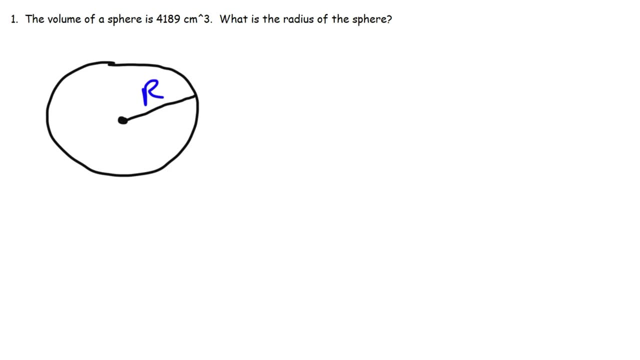 Now the formula that applies to this equation is this: The volume is equal to 4 thirds pi r cubed. Now we can plug in the numbers at this point and solve for r, or we could rearrange the equation and just plug in and get the answer directly. 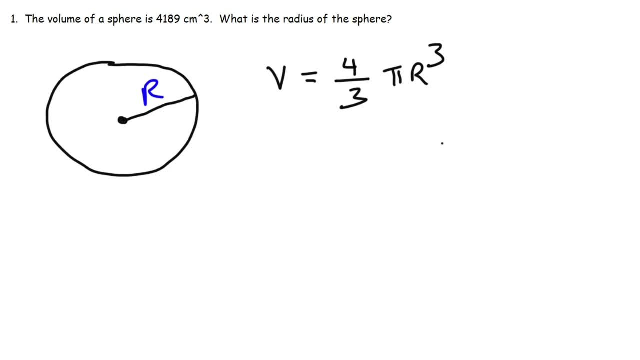 Let's do it that way. Let's solve for r. So first I'm going to multiply both sides by 3. These will cancel. So I have: 3v is equal to 4pi r cubed. Next I'm going to divide both sides by 4pi. 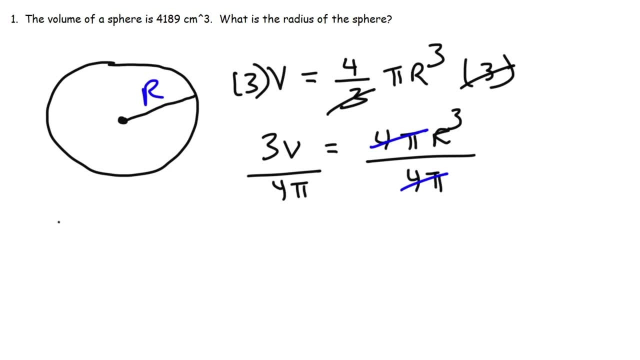 So now what I have is 3v over 4pi is equal to r to the third power. Now to get r by itself I need to raise both sides of the equation to the 1. Or take the cube root of both sides. 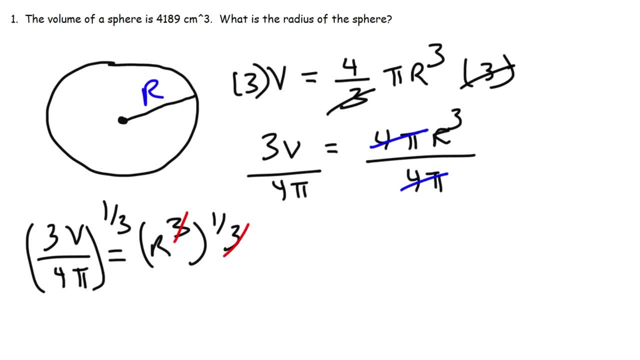 3 times 1 third is 1.. So we're going to get this formula: The radius of the sphere is 1 third, which is equivalent to being the cube root of 3 times the volume of the sphere divided by 4pi. 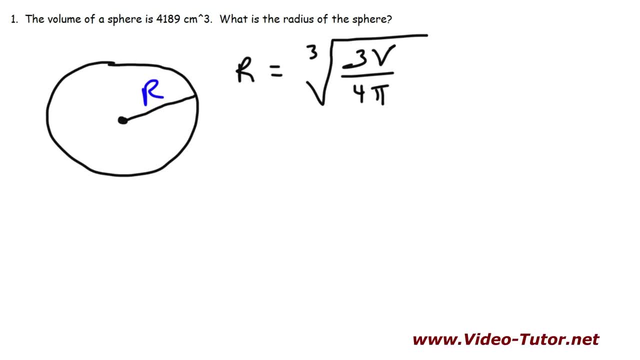 Now let's go ahead and plug in everything into the equation. So this is going to be 3 times 4189 divided by 4pi, And I'm going to use the exact value of pi in the calculator. By the way, make sure to put this in parenthesis, otherwise you could get a different answer. 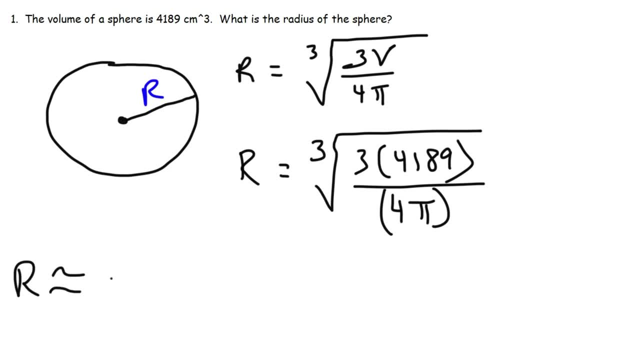 So the radius of the sphere is approximately 10 centimeters And you could determine the unit based on what we see here. So that's how you can calculate the radius of the sphere, given the volume. Alright, let's try another example. Feel free to pause the video if you want to work on this example. 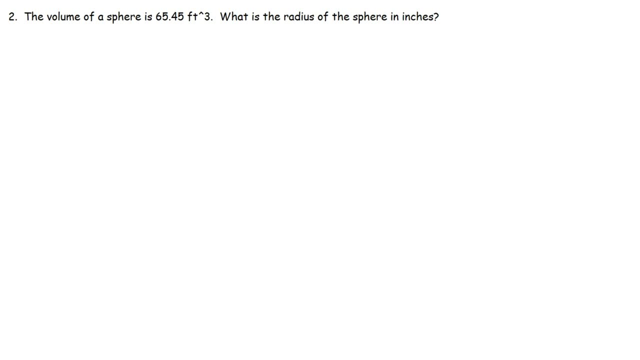 So we're given the volume of the sphere- this time it's in cubic feet- And we need to find the radius of the sphere, but in a different unit, in inches. So what we're going to do in this problem is we're going to calculate the radius first. 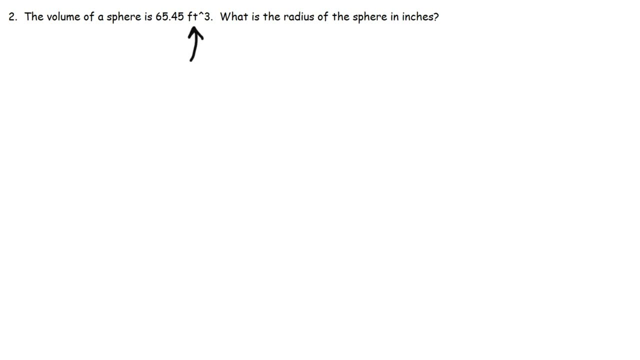 And it's going to be in the same unit that we see here. It's going to be in feet, And then we'll change the unit from feet to inches, So let's use the formula, The formula that we used in the last problem. 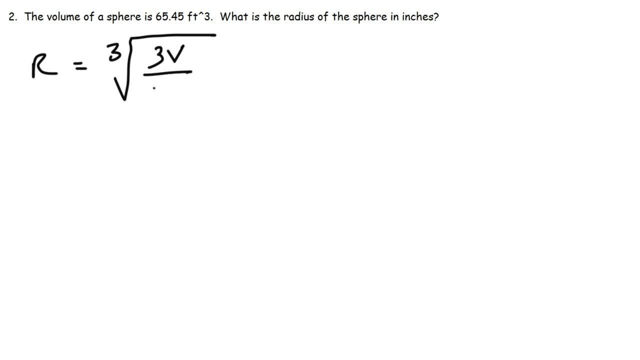 The radius is equal to the cube root of 3 times the volume divided by 4 pi. So let's replace v with 65.45 cubic feet. We'll talk about the units as well, Divided by 4 pi, And let's use the exact value of pi. 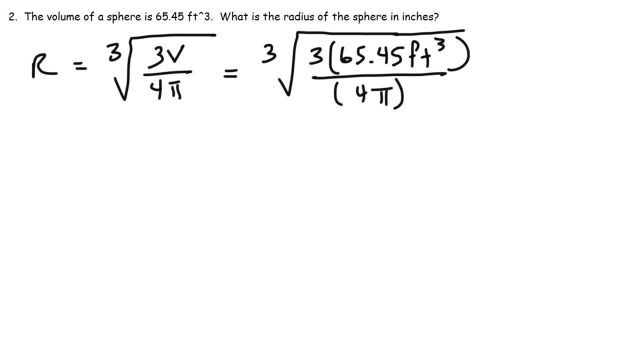 So you should get that. r is approximately 2.5.. Now notice that we have the cube root of feet cubed. So when you take the cube root- I'm just going to write it here real quick- If you take the cube root of feet cubed, the threes will cancel. 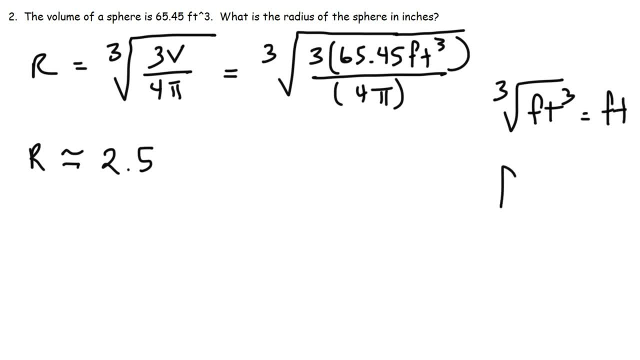 So you just get the unit feet. This is equivalent to raising this to the one-third power. Three times one-third is just one, So the radius is just going to be just feet, Not feet squared or feet cubed. Now that we have the radius of the sphere in feet, let's go ahead and convert it to inches. 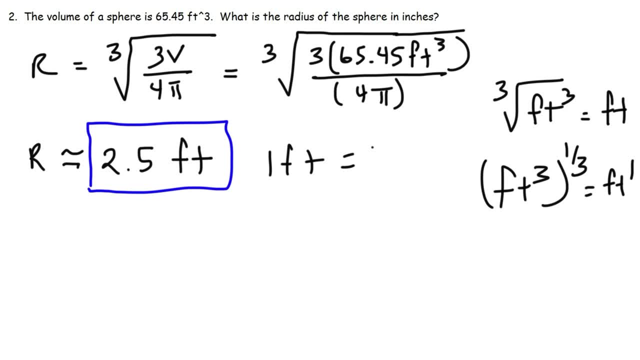 Now keep in mind there's 12 inches. 12 inches and a foot, So that's our conversion factor. So let's start with what we have, And then in the next fraction, we'll write 12 inches per foot. We'll write it in such a way that the unit feet will cancel, leaving us with inches.